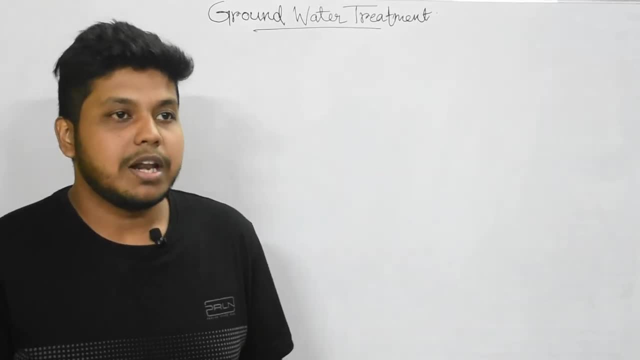 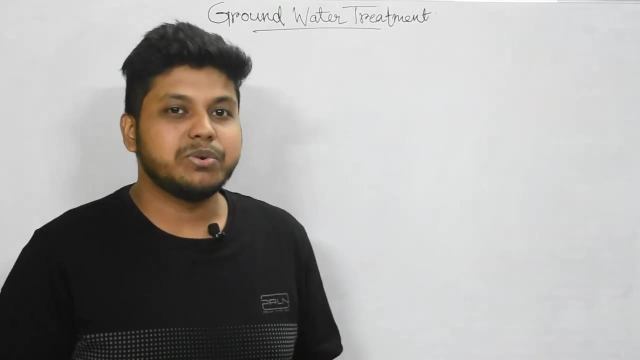 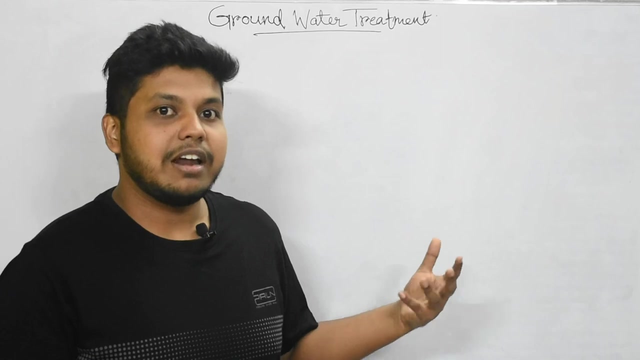 turbid free and they are pathogen free like uh. there is no pathogenic bacteria in general- but in that case that groundwater can be treated by providing some minimal doses of chlorine, that is, that is a disinfection process, and then it can be supplied to the domestic purposes. so in 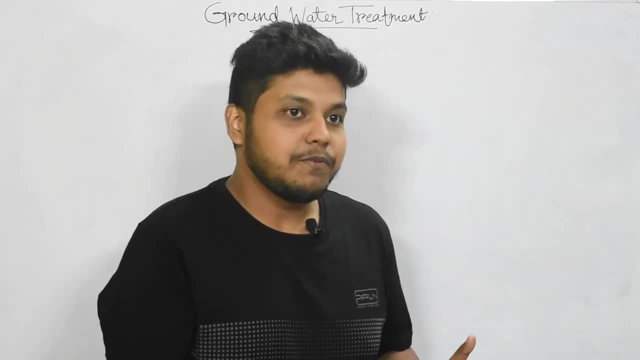 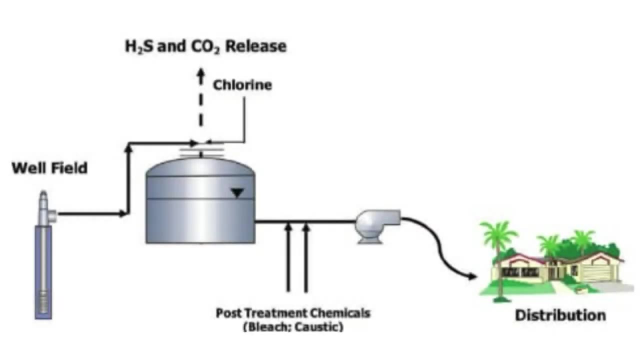 let us see a example by a pictorial presentation for this case study. so uh, this picture shows the pathogen. free groundwater can be treated like this here. this is a disinfection process where chlorine is added and the dissolved gases like co2, h2s, is released from there. 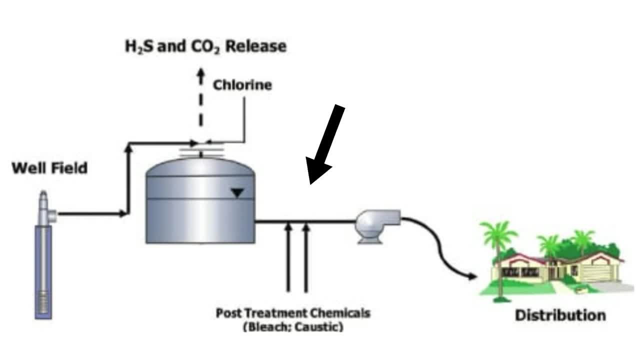 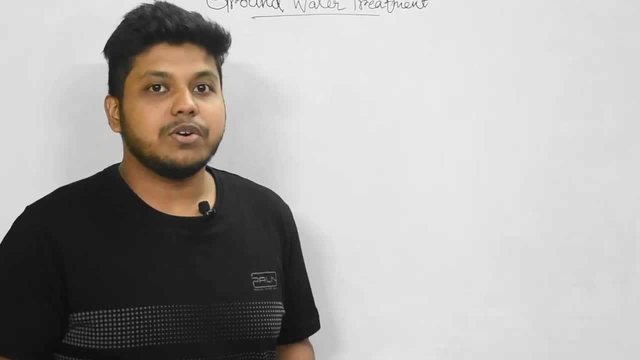 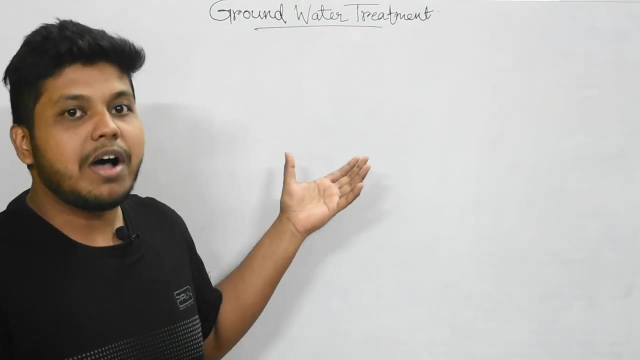 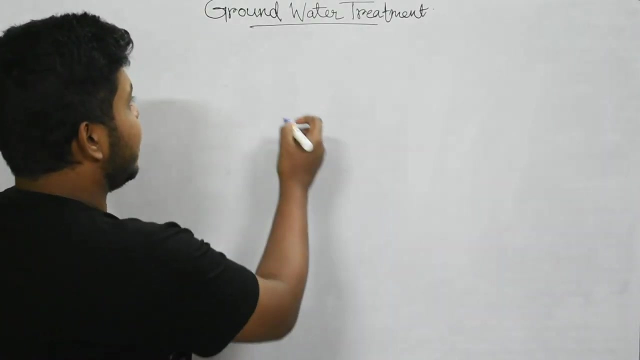 and after that. this is a post-climation process to erase the further contamination from the distribution system. so now we will discuss the groundwater which have some contaminants or some organic materials. so most of these cases the presence of, and manganese which can be removed from this groundwater is by the process of aeration. so the 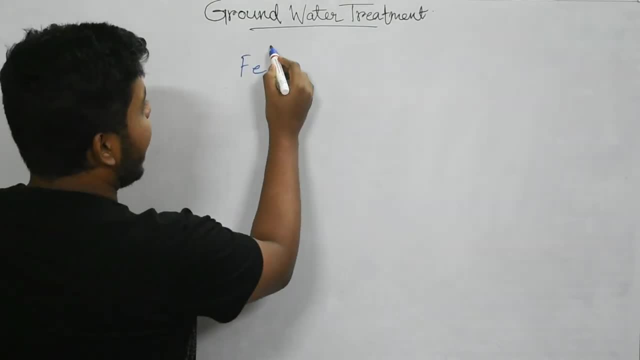 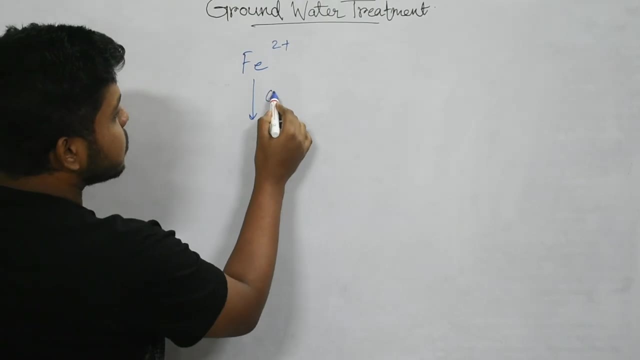 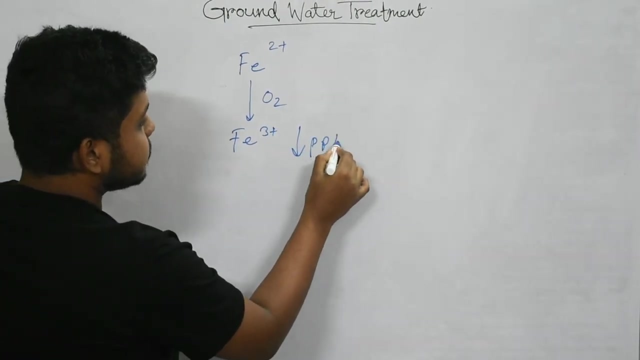 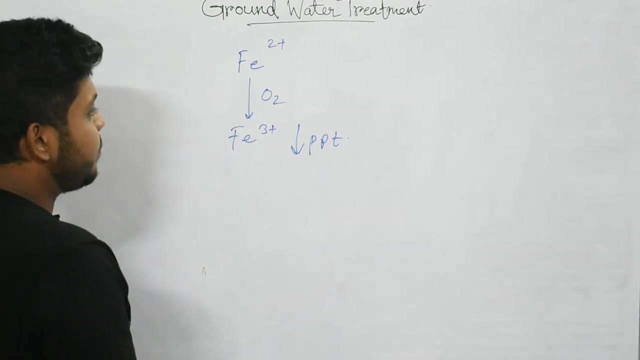 fe, that is iron, in the groundwater is present as fe2 plus, so this is in the dissolved form. so if the aeration process happened, so in presence of oxygen it gets fe3 plus precipitation. so in this way this iron can be removed from this groundwater treatment. now another one. there are 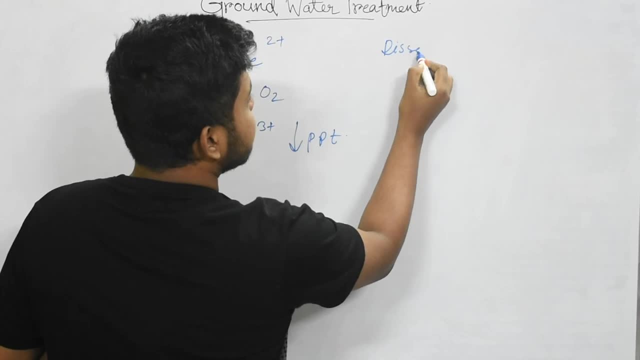 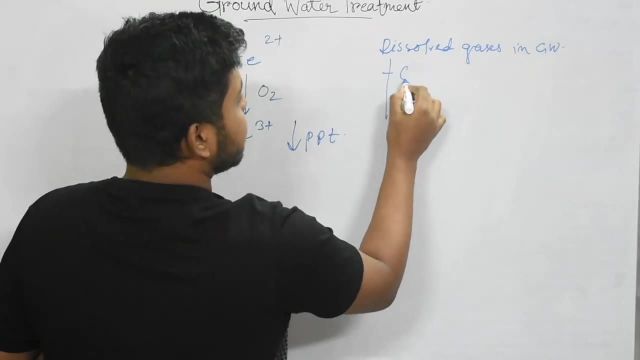 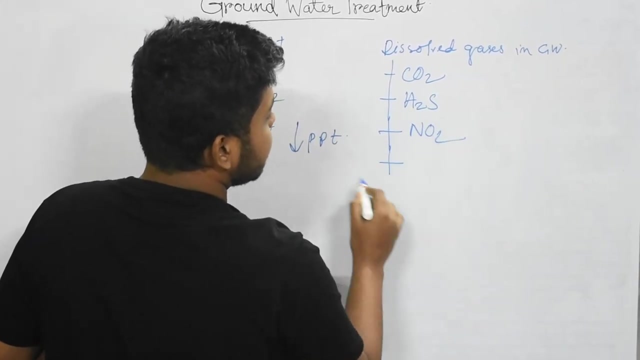 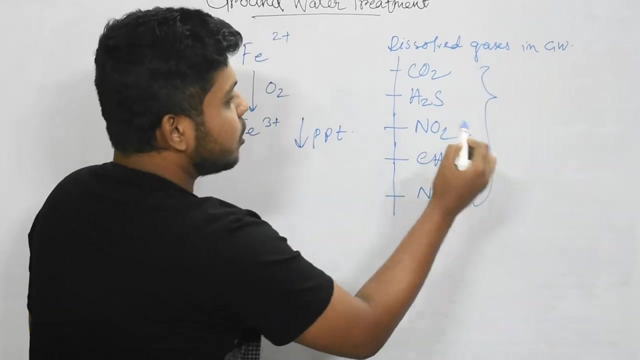 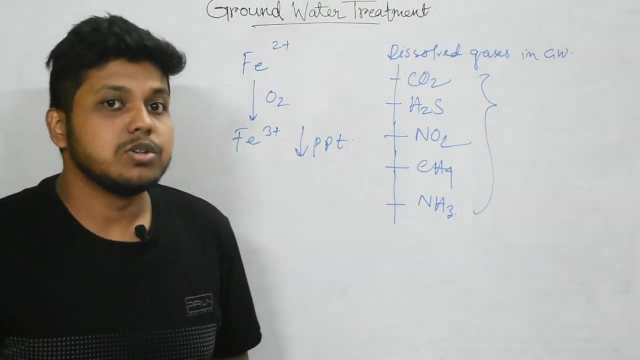 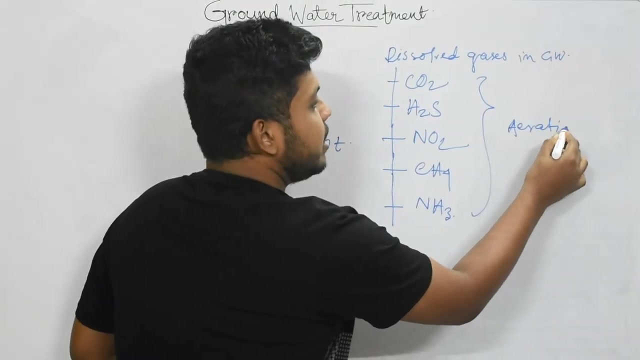 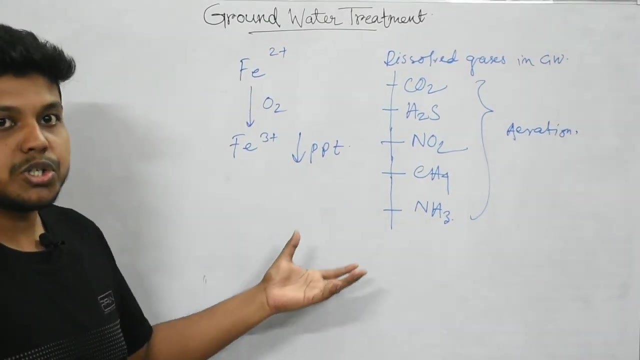 some dissolved gases. dissolved gases in groundwater. they are like co2, h2s, nitrogen oxide, methane, ammonia. so these dissolved gases causes bad odor, bad taste and some corrosivity in the groundwater. so this can be omitted from this groundwater by the process of aeration. so we will discuss this aeration process in detail in our next lecture. so let us see a flow chart. 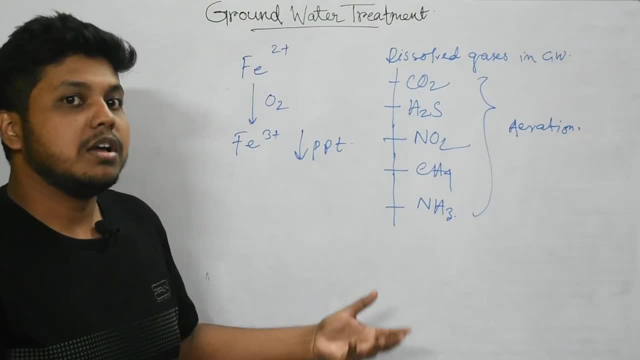 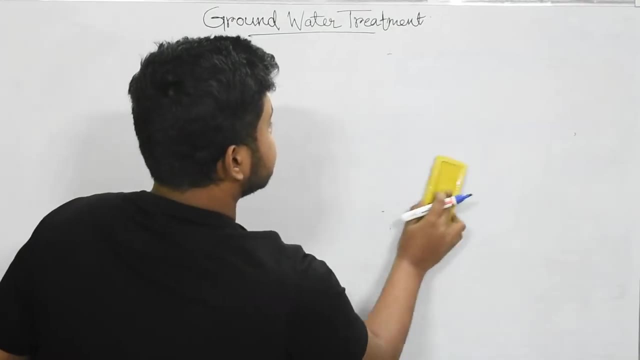 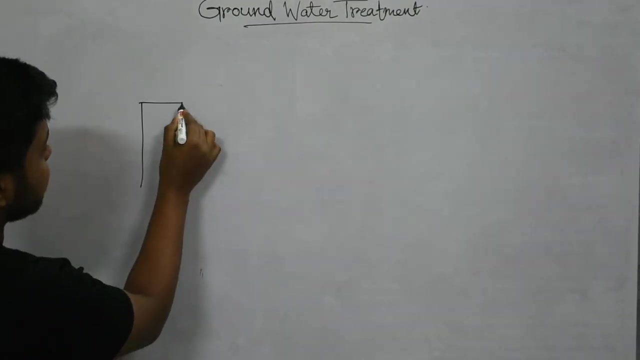 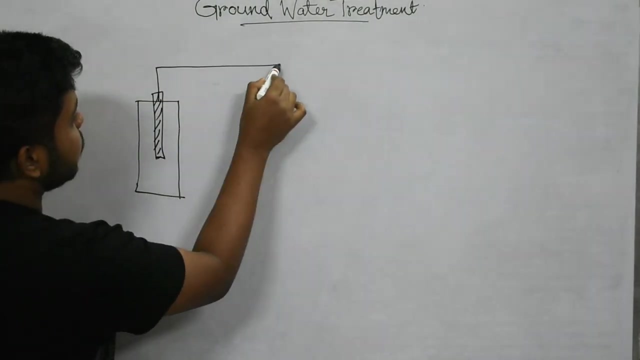 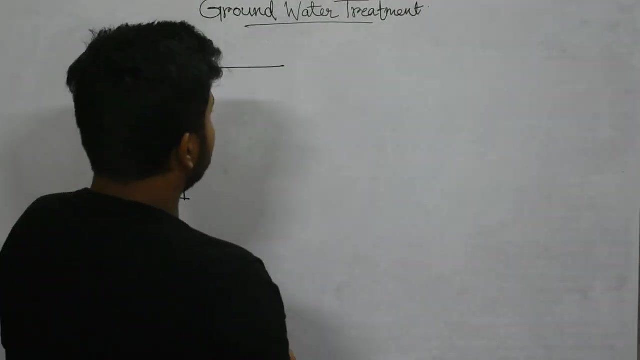 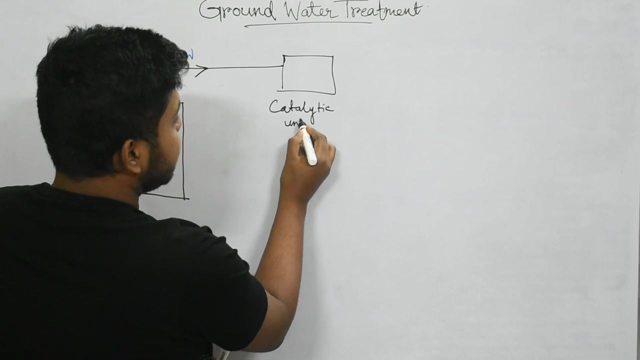 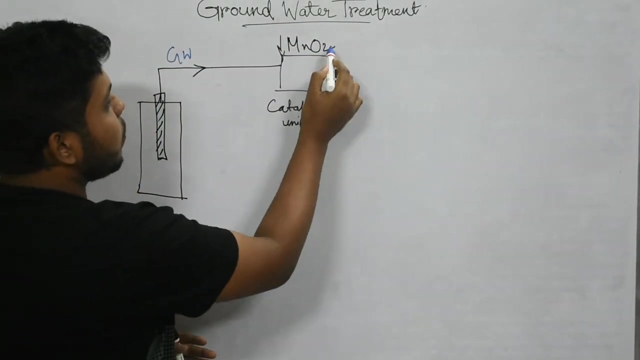 that will show how the groundwater treatment happens in some different unit processes. so if this is a tube well from where the water is pumped, so this is ground water pumped through from this tube well, so a catalytic unit. this is a catalytic unit, here MnO2 catalyst. it's provided here, so why this is provided. 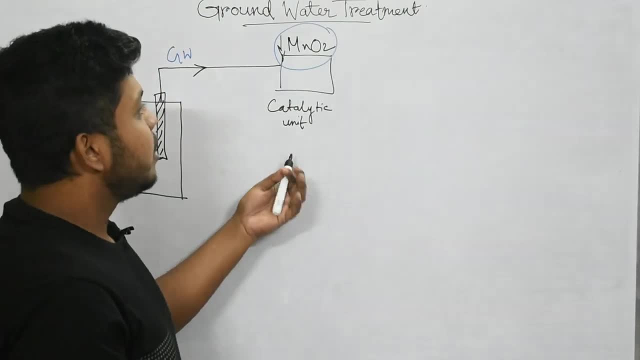 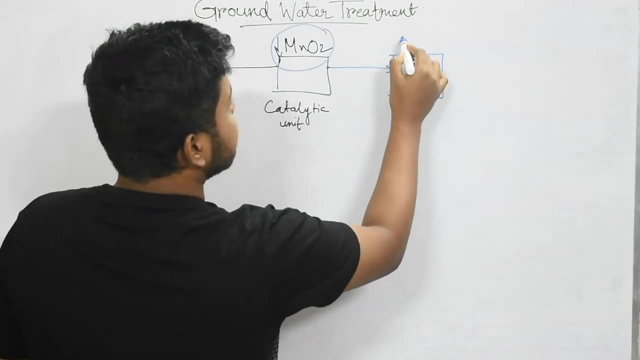 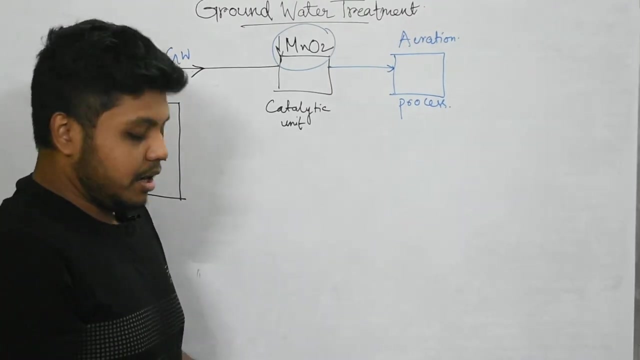 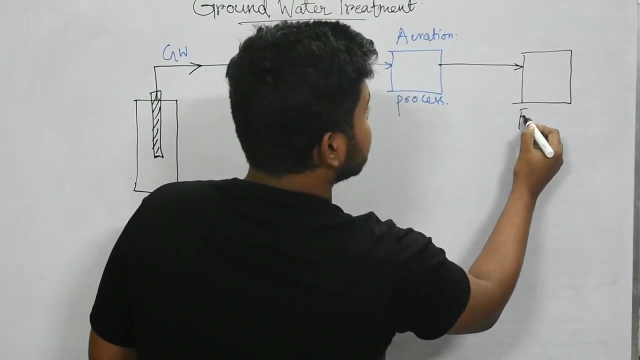 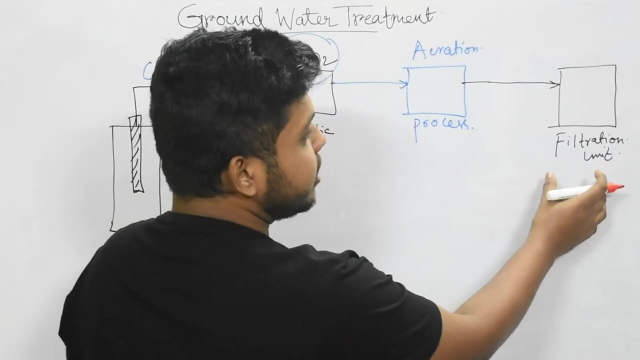 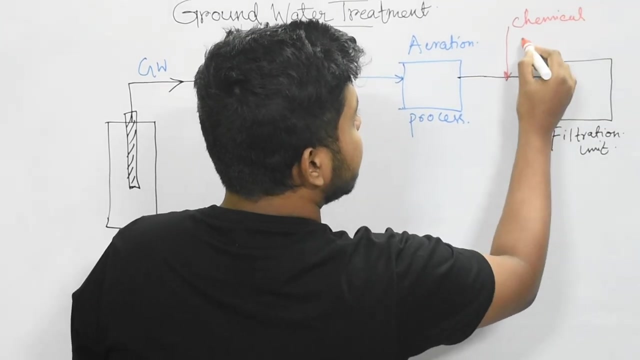 to increase the rate of reaction or to minimize the time requirement for this aeration process. so after that, the aeration process. aeration process is provided now. after this, the water sent to filtration unit. now, before this filtration unit, we can have here addition of chemical coagulants like alum. so here, 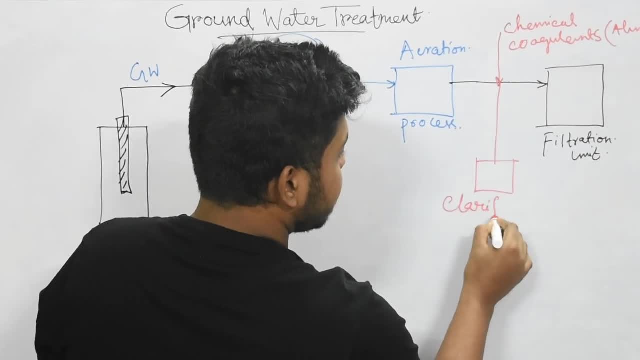 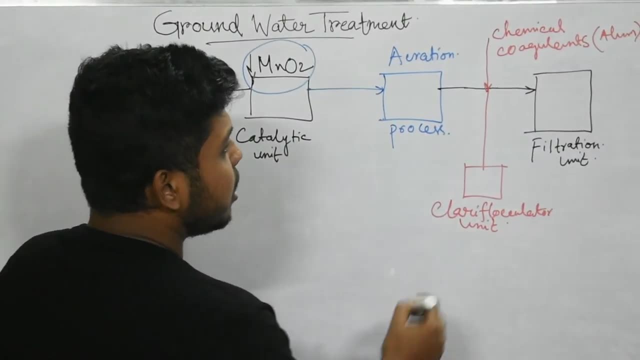 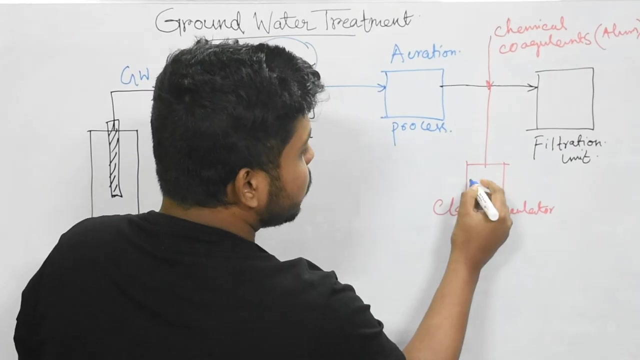 a clariflocculator unit is provided. that is chemical sedimentation because after this aeration process, the suspended solids and the colloids. this can be removed by adding this coagulants, by forming some flocs and as removing as sludge from here. so after this, 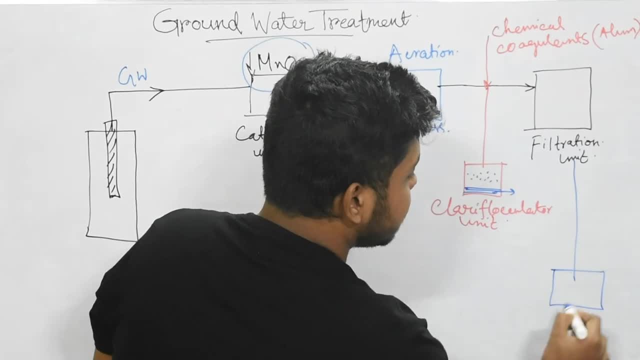 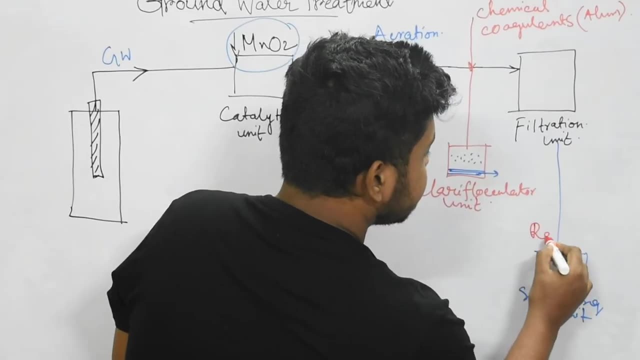 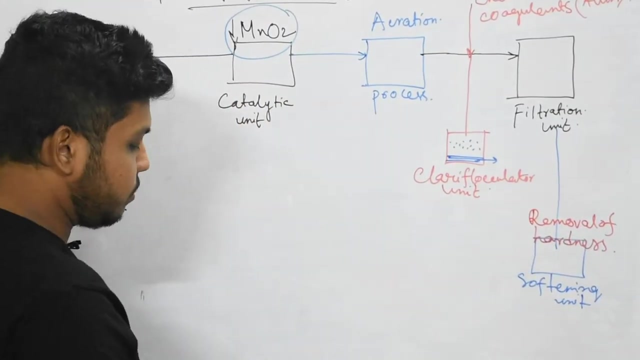 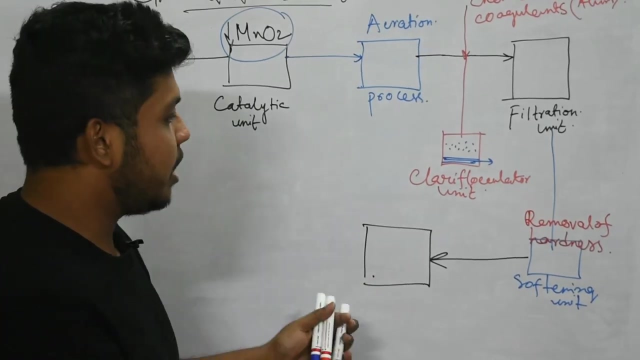 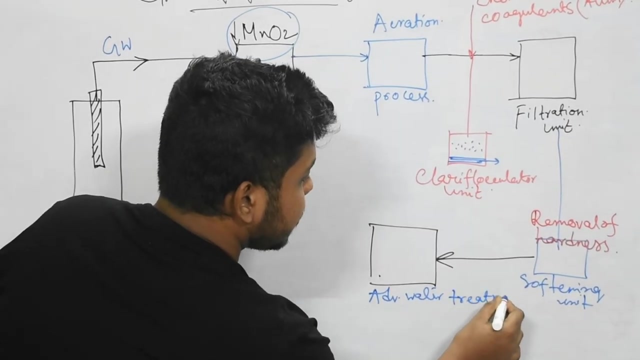 filtration unit, there is softening unit for removal of hardness. if this water has some hardness, this can be removed by this softening unit. now, after this, the advanced water treatment system can be provided. so this is advanced water treatment. so this can be provided in the form of ro, that is, reverse osmosis.